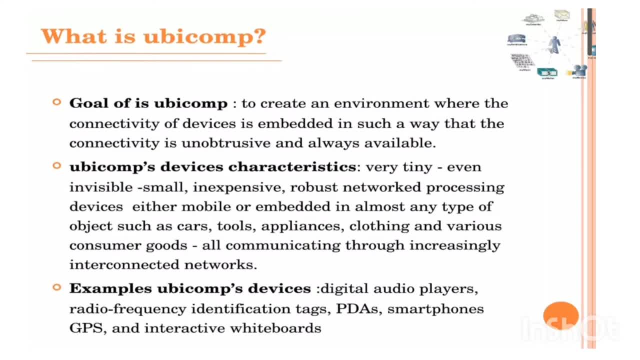 Goals of Ubicom To create an environment where the connectivity of the devices is embedded in such a way that the connectivity is unprettious and always available. Ubicom devices characteristics: They are tiny, even invisible. small, inexpensive, robust network processing devices, either mobile or embedded in almost any type of objects, such as cars, tools, appliances, clothing and various consumer goods also communicating through an increasingly interconnected network. 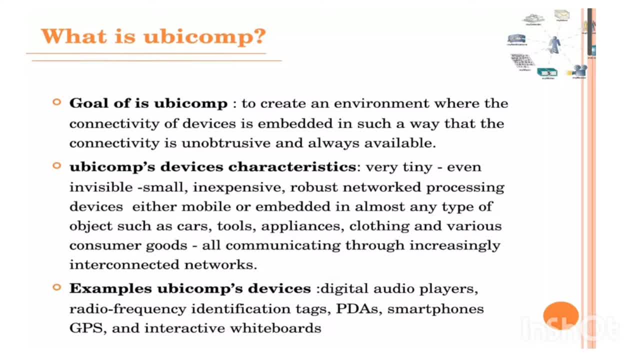 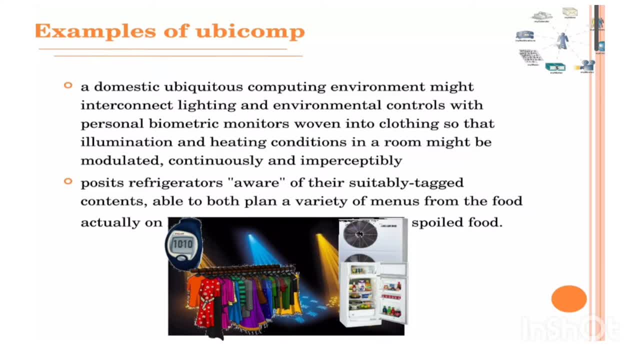 Examples of Ubicom devices are PDAs, smartphones, GPS, digital audio player, etc. Examples of Ubicoms are A domestic ubiquitous computing environment. might interconnect lightly an environment control with the personal biometric monitors and woven into a clothing so that the illumination and heating conditions in a room might be modulated continuously and imperfectly. 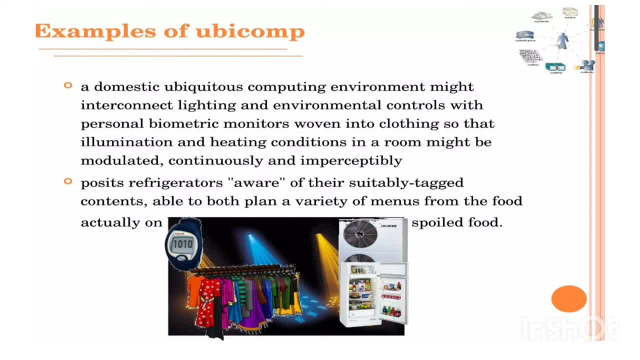 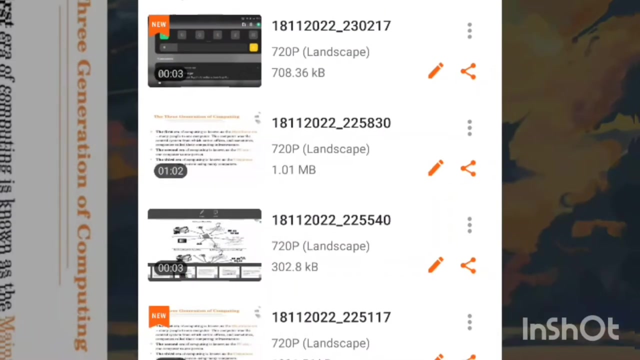 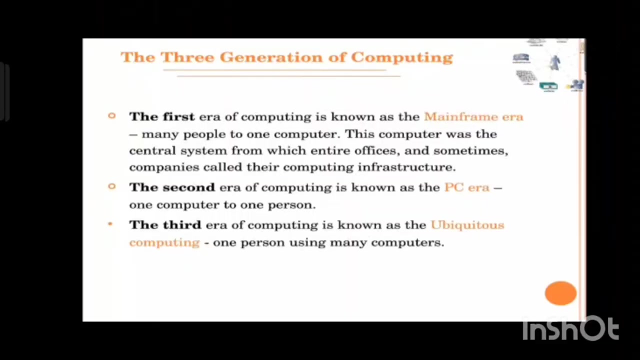 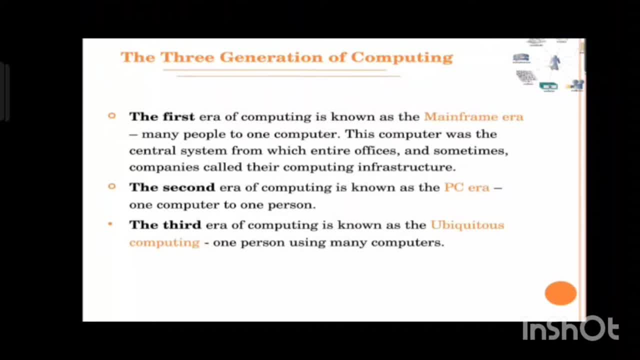 computing. The first generation, that is the first era of computing, is known as the mainframe era. In this era many people uses one computer, That is, this computer system was the central system from which entire offices and sometimes companies call that infrastructure. The second era of computing, that is, the second generation, is known as PC era, in which one 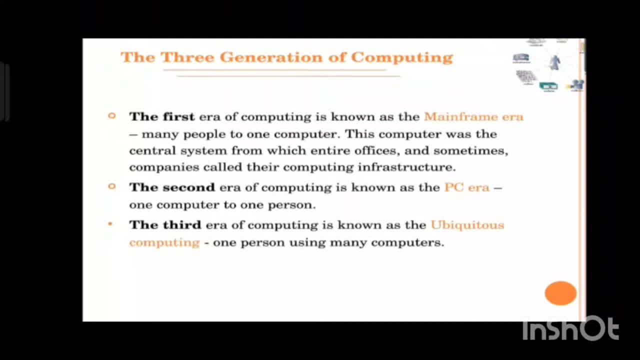 computer uses one person, That is, a person can own his own computer. The third era of computing is called as ubiquitous computing, in which one person can access many computer system. In this third era, the workload has been distributed, That's why the tasks are made easier. 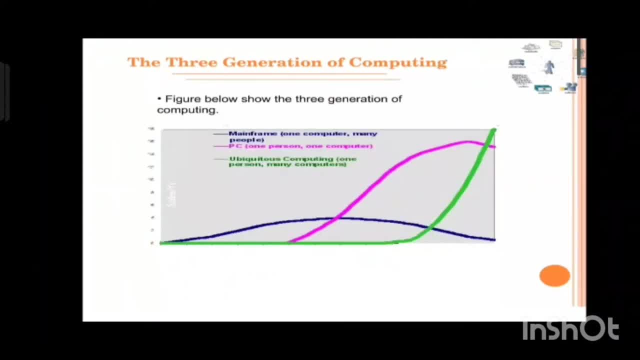 The figure given below shows the Zigbee system, Cutting out the 4 components from the bigger structure. cutting out the bottom, thats two components. This one is called the floating form and what a supporting piece is. this one is called company room. shows the generations of computing. the blue line indicates the mainframe era. 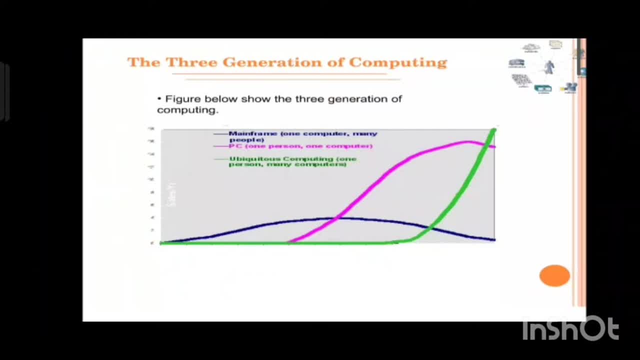 that is one computer and many people in this. in this era the workload was much more on the computer system. in the pink line indicates the one person, one computer. that is PC era. it was moderate. and the third one that is ubiquitous computing is indicated by green line where one person can access to many. 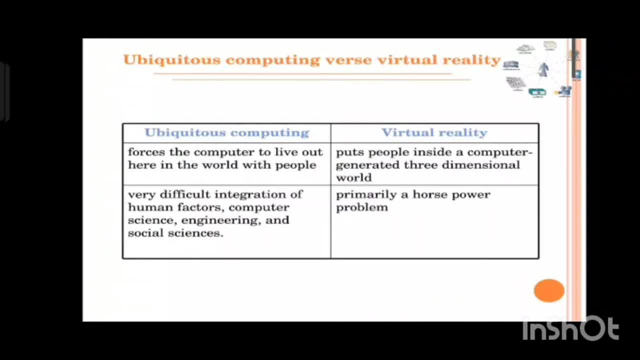 computers. this next is ubiquitous computing. was ubiquitous computing versus virtual reality? your ubiquitous computing is basically about bringing computing to people's physical world and integrating the physical world into the physical world and integrating the with everyday objects and activities and making comfortable with a human world. and virtual reality is totally opposite, that is, it is about simulating physical 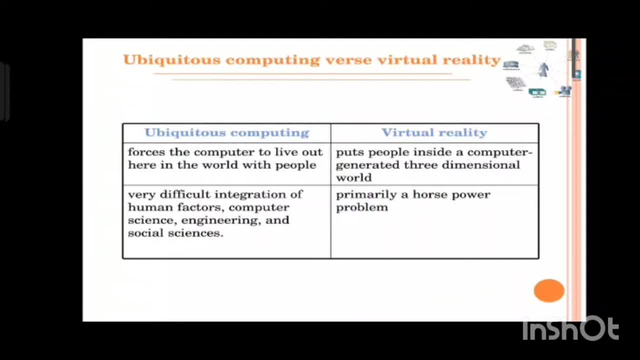 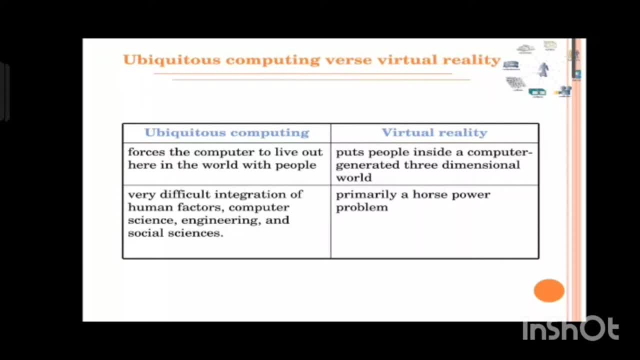 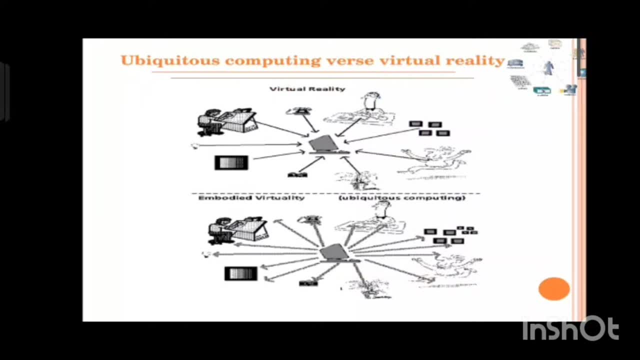 virtual reality is primarily a horsepower problem. ubiquitous computing versus virtual reality in this picture. the first picture predicts the virtual reality, whereas the second one gives us the you- biquitous computing that is also known as embodied virtual reality- that Dreidman was taking on in ok. 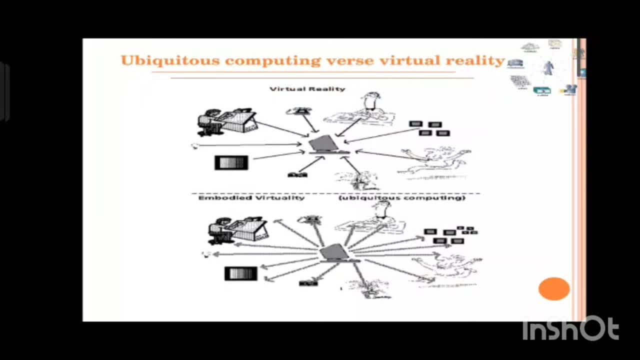 tablets. we need a 서버 would be perfect. so digital reality, as you wanna process the mac to perfectly circular, thou q см prima cic and not harvest a virtuality, and first one, many, many people, or the many people or human resources, has to be the part of computer, that is, they are mainly dependent on the 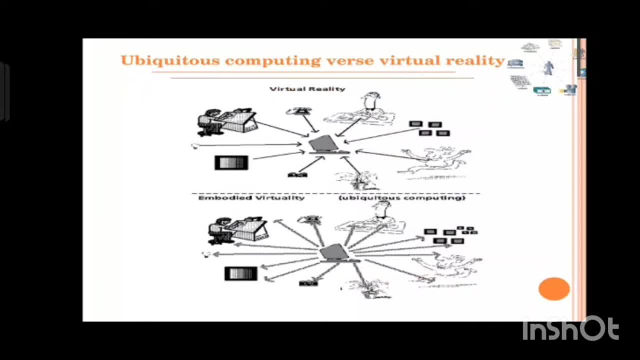 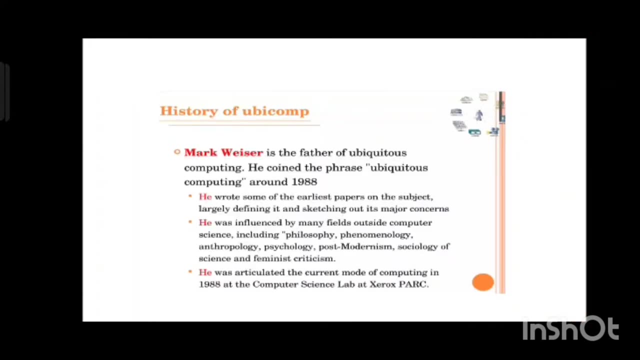 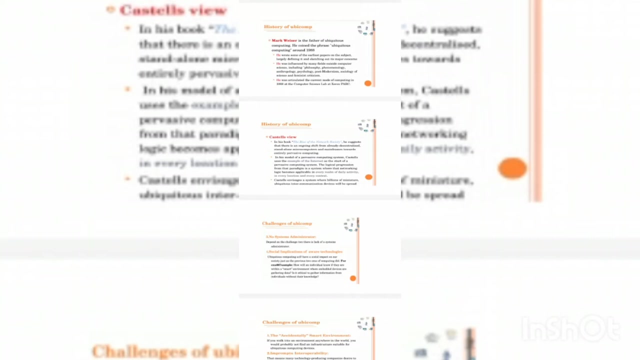 computer system which has limited applications and accesses, whereas ubiquitous computing, the computer itself becomes the part of human world. thank you, hi. I didn't call in history of you become. marks Wieser is of other of ubiquitous computing, his coin in the Fraser. ubiquitous computing around 1988. 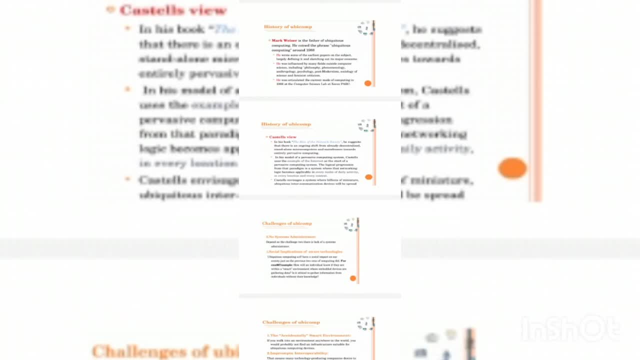 he is written some of the earliest paper on the subject largely defined its- and sketching now you its- major concern. He was influenced by many fields outside computer science, including philosophy, phenomenology, anthropology, philosophy, postmodernism, sociology of science and 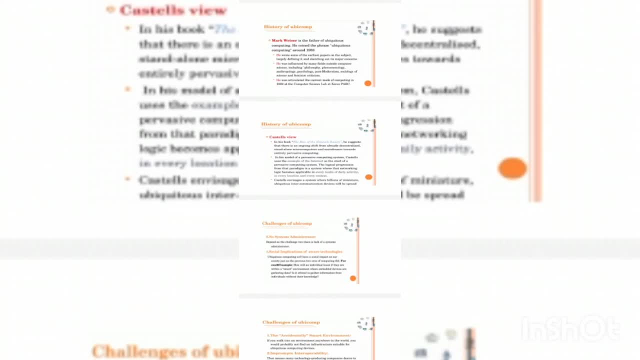 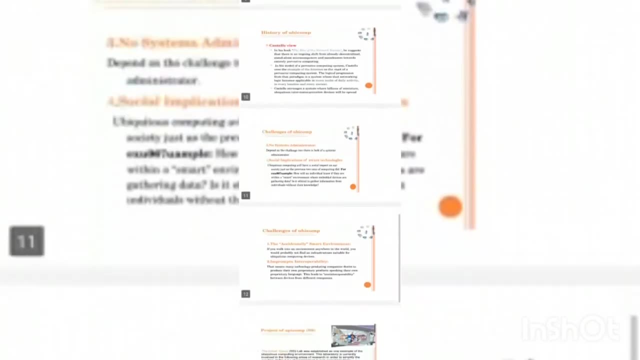 feminism. He was articulated the current mode of computing in 1988 at the computer science lab at Xerox PARC Castel view. In his book The Horizon of the Networking Society he struggled. There is an ongoing shift from already decentralized and along microcomputer. 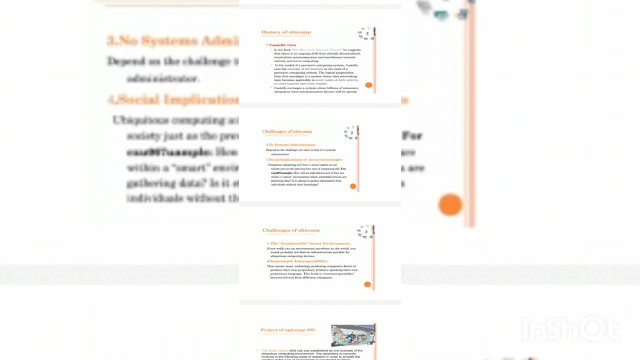 and meant from toward entire pre-wised computing. In his model of previous computing system, Castel used the example of the internet As the start of the pre-wised computing system. the logical progression from that programming is a system where the networking logic becomes an application in every realm of daily activities. 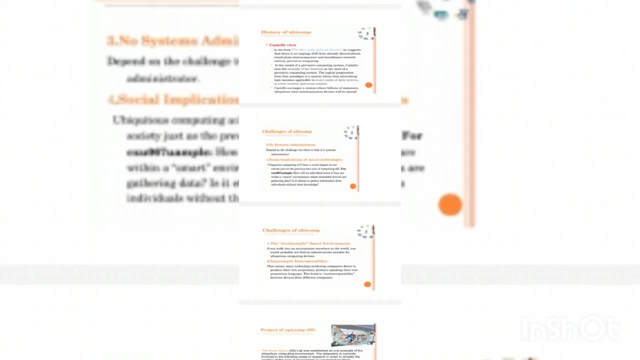 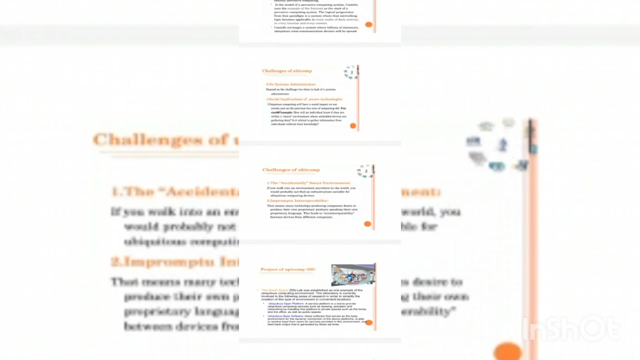 in every location and every context. Castel, even a generational system where millions of manufacturing ubiquitous intercommunication devices will be spread. Number system: The administration depends on the challenges too. There is a lack of a system to administer the social implications of our technologies. Ubiquitous computing will have a social impact. 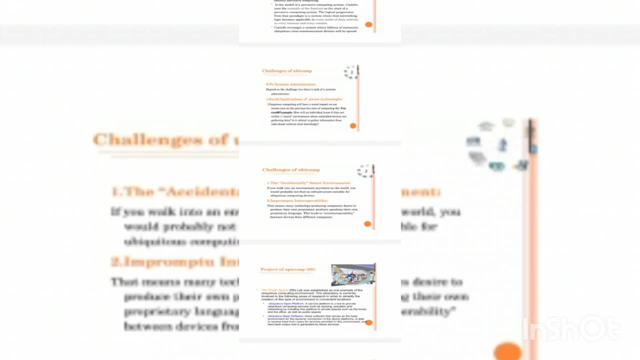 on your society, just as the previous two early of computing did. for how will be individual known if they are within a smart environment where embedded devices are gathering data? Else it is not ethical to gather data Else it is not ethical to gather information from individuals without their knowledge. 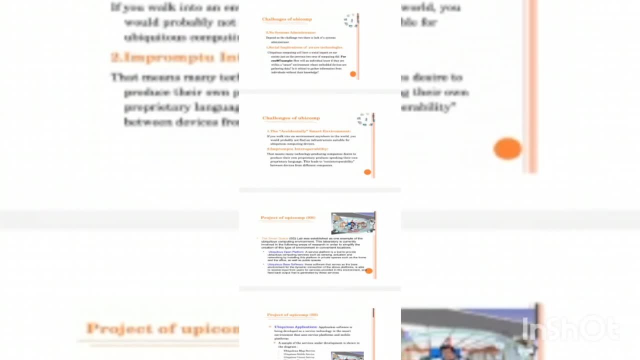 The accidental smart environment, If you walk into an environment where in the world you will probably not find an infrastructure suitable for ubiquitous computing devices' interoperability, that means many technology-producing devices, The new technology-producing technology, the new technology-producing technology, the new 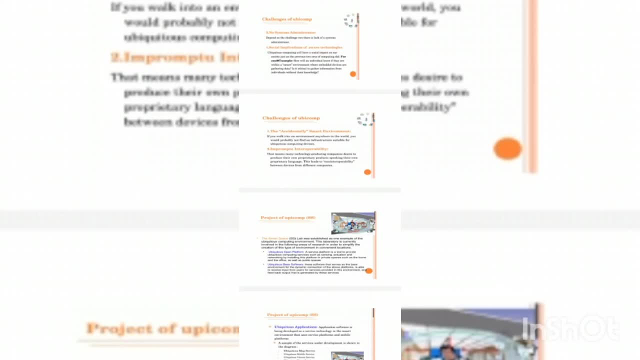 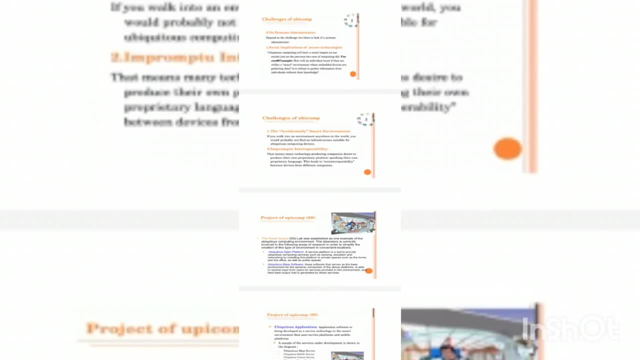 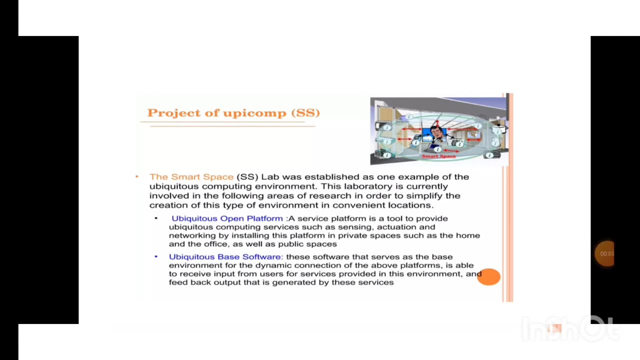 the third generation. Also, therices have been 영상을 hands-on. The pathway onto the future. Thank you, My name is Cheom's team. I am a My name's Knowbeck. UBICOM is if a home office is built around the dimensions of the current. 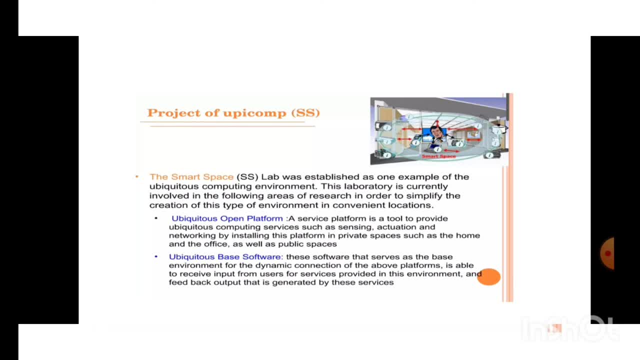 in the following areas of research in order to simplify the creation of this type of environment in convenient locations. first: ubiquitous open platform. a service platform is tool to provide ubiquitous computing services, such as sensing, accreditation and the networking, by installing this platform in private spaces such as home and office, as well as public spaces. second: ubiquitous 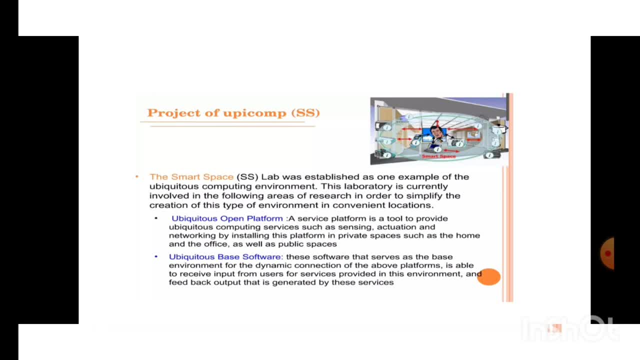 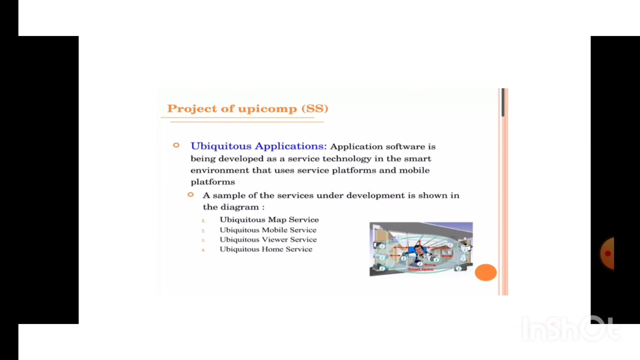 base software. this software that serves as the basis moment for the dynamic connection of the upper platform. he's able to receive input from the user for services provided in this inform environment and feedback output that is generated by these surfaces. next, ubiquitous application: application software there is been developed as a service technology in the smart environment.